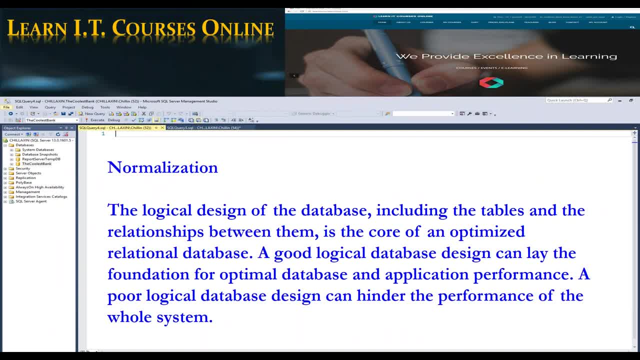 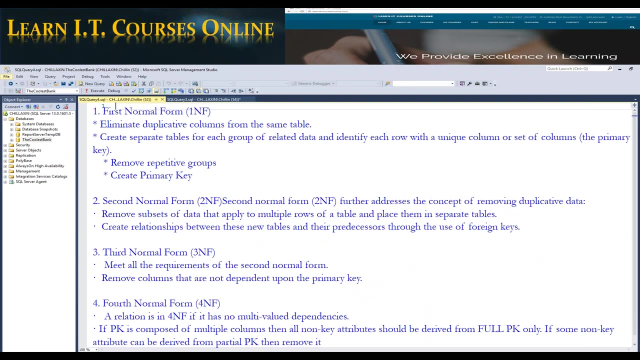 So that concept became known as normalization. Normalization is the logical design of the database, including the tables and the relationships between them, to ensure that we have an optimal or optimized relational database. One thing that's definitely going to come in an interview if you're applying for a data modeler or database administrator's position on database design is: what is normalization and what are the different forms. 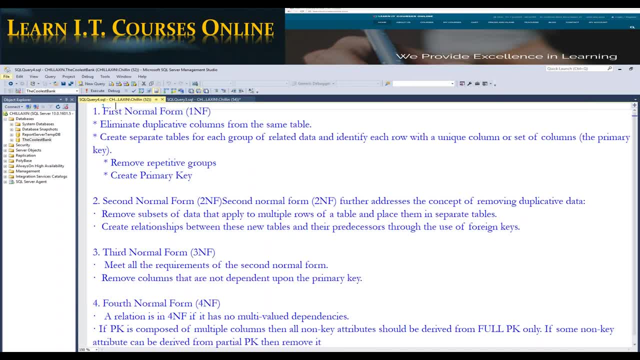 or levels and forms of normalization. And that's where we get into the different levels: The first, normal form, the second, the third, the fourth, describing that with the first one we eliminate any duplicate columns from the table, And then the second one, we remove subsets of data that apply to multiple rows. 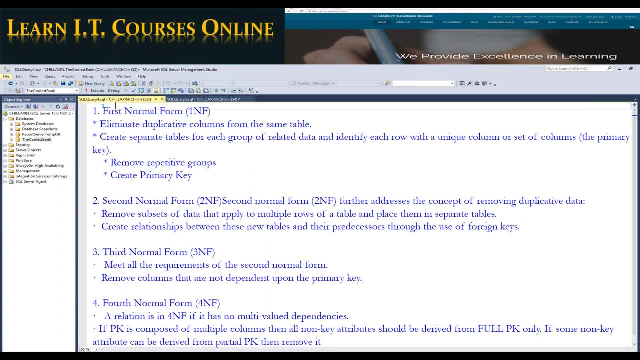 And then the third one- remove columns that are not dependent upon the primary key- And then the fourth one. a relationship in the fourth normal form has no multivalued dependencies, So those are the kind of things that we're going to be looking at in the next few weeks. 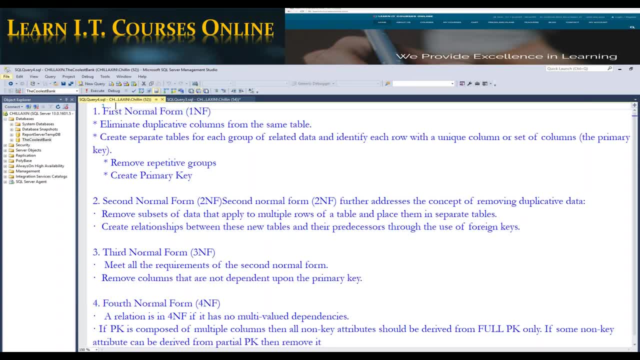 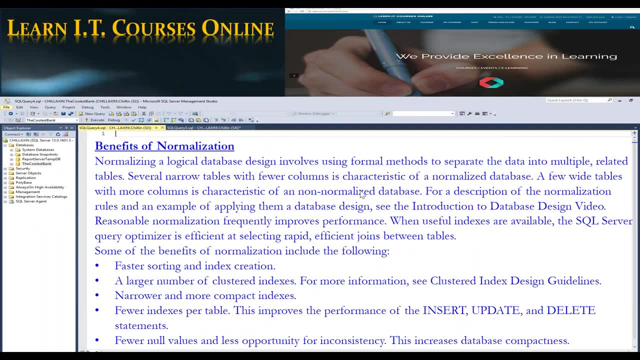 Those are the kind of things that we need to have practiced and memorized so that we can go to an interview and definitely be able to answer anything that's normalization-related. And, of course, what are the benefits? And then there are a few benefits. 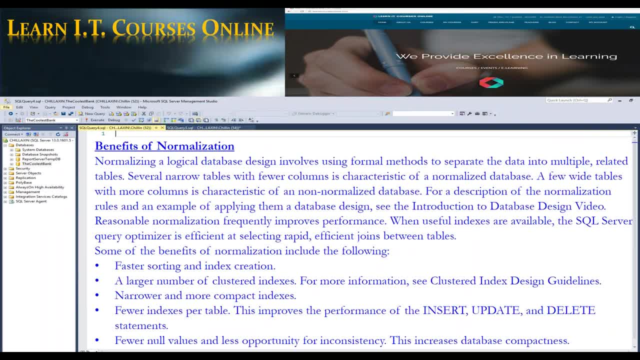 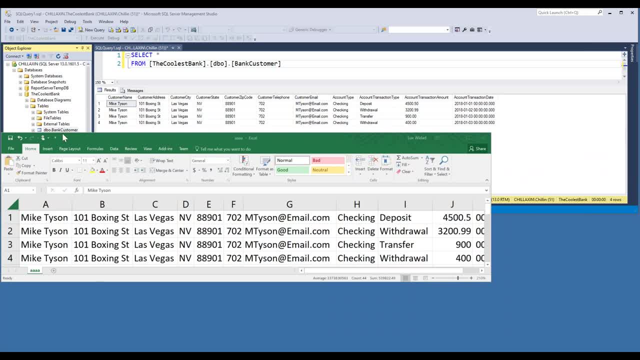 So you can see a database called The Coolest Bank And then there's a table called Bank Customer. And as I select all the records, the four records that we have in there, we have our customer's name, Mike Tyson, who lives in 101 Boxing Street in Las Vegas, Nevada. 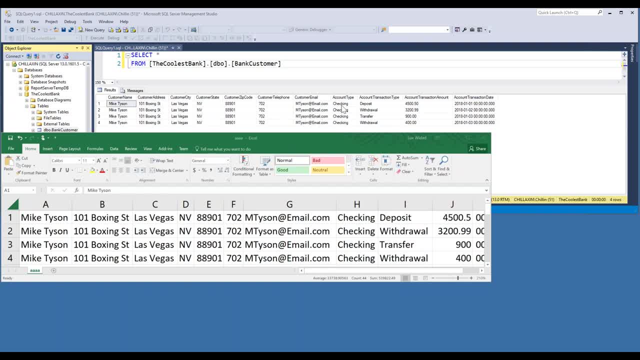 Zip code: 88901.. Area code: email account type: He has a checking account with us. Here's the transaction. So they've had a deposit, a withdrawal, a transfer, a withdrawal, and then the amounts Of each transaction. 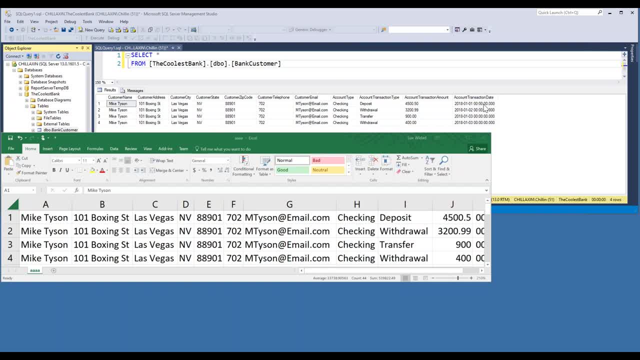 And then the dates, So on January 1st of 2018, January 2nd of 2018, and on January 3rd, there's actually two transactions- Transfer and a withdrawal- And I have the same information in Excel. 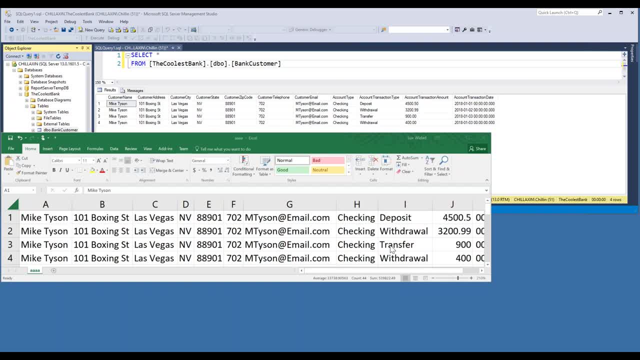 In Excel. this is something that we might find, And that's what we call a flat file, where everything is just stored in one big fat file that has all the information. So, as we notice, there is a number of things here. The first one is: you would see that there's some information that changes. 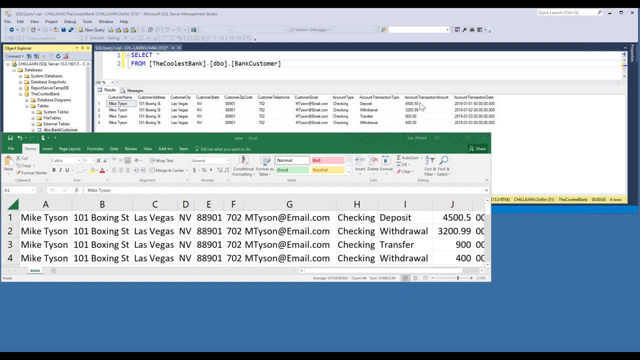 So with each transaction I'm having different amounts: $4,500, $3,200, $0.99,, $900, $400,. transaction type might change: deposit withdrawal, transfer withdrawal. the dates change But notice with each entry the name repeats because it's for the same person. 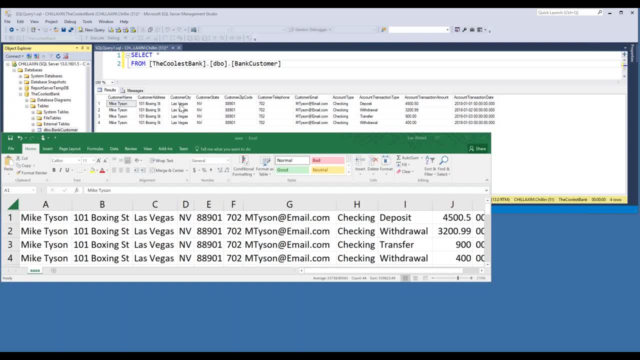 The address repeats because it's for the same person. The city is still the same, Related to the address, the state, the zip code, the telephone number. So the first thing that happens in the relational database, because in the relation database, unlike a flat file, in a flat file if I was to have two Excel sheets or two flat files, there's no way I can go into one file and pull in information and relate it to another one. 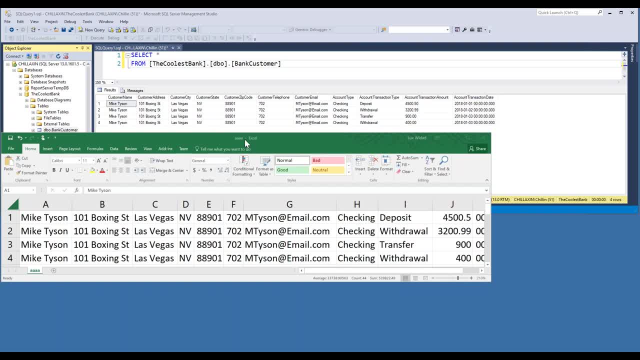 But in a relational database I'm able to have multiple files And when a file is stored in a database it's called a table. I can have multiple, I can have multiple tables and I can have a relationship between them, So it's very easy for me to get that information from one table that's related to another table, as long as I've built that relationship between them. 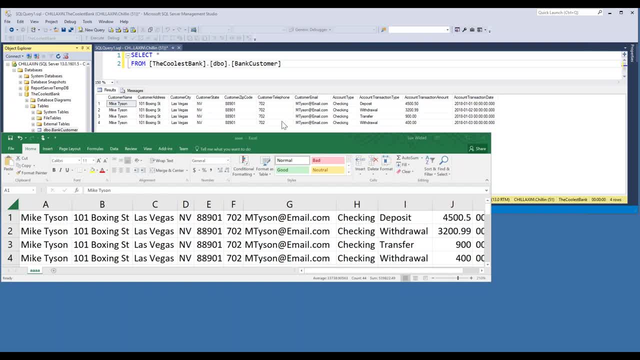 So it then makes sense for me to, instead of repeating this information over and over for each new entry, for each new transaction, that I can have it one time, in one place, in one table, all by itself. So the first thing is not having duplicate data. 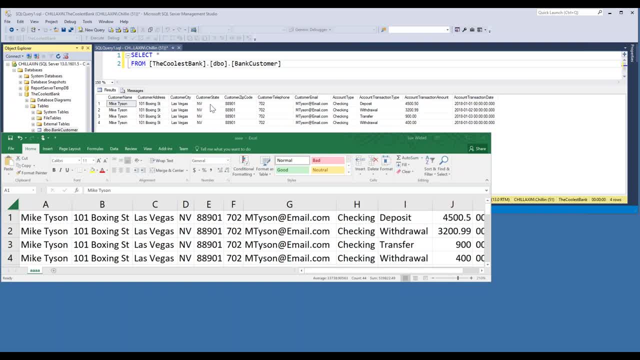 There's a lot of advantages for not having duplicate data. For instance, just to oversimplify it, let's assume that each letter that's stored in the database takes one meg, just to oversimplify the numbers. So if I was to have Mike Tyson, that's 1, 2, 3, 4, including the space 5, 6,, 7,, 8,, 9, 10.. 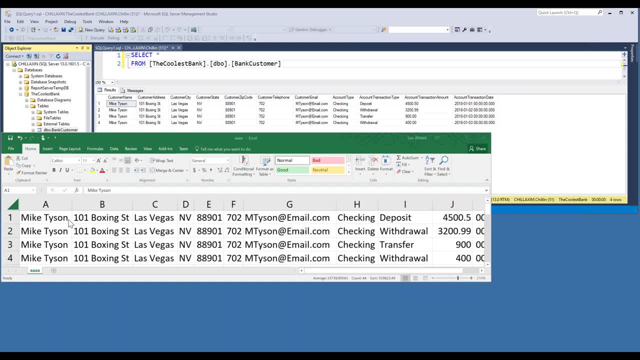 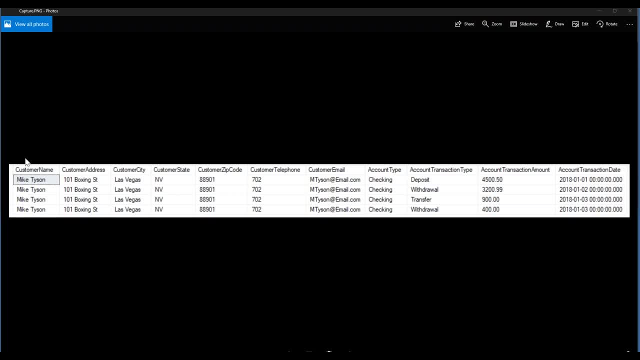 And then I multiply that by all this information, that's all duplicates. all this information be grouped together. Notice that the first column is the customer's name, so it's customer-related. The second one is the customer address, so it's again customer-related. The customer city where 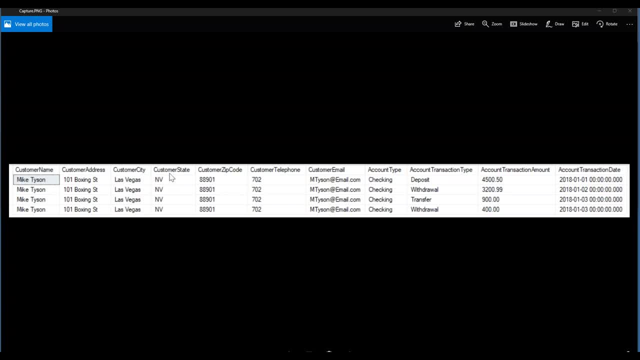 they live. so it's customer-related. The customer state, which is kind of related to the customer as well, and then the customer zip code, where they live, their residence, and the customer telephone number and customer email. So all this information links back to the customer. 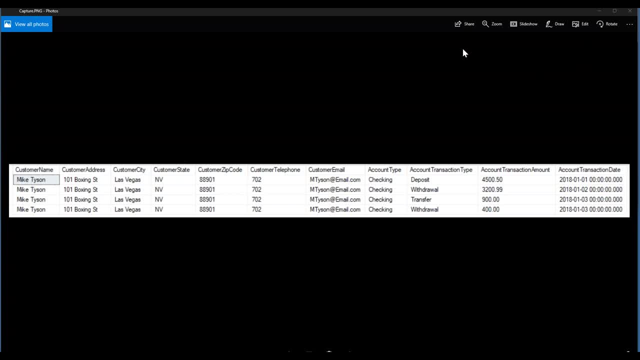 The second thing is, or the second group of columns relate to something else. Well, we have an account type, so this is kind of account-related information: The account transaction type, which again is kind of related to the account. The account transaction amount, which again is: 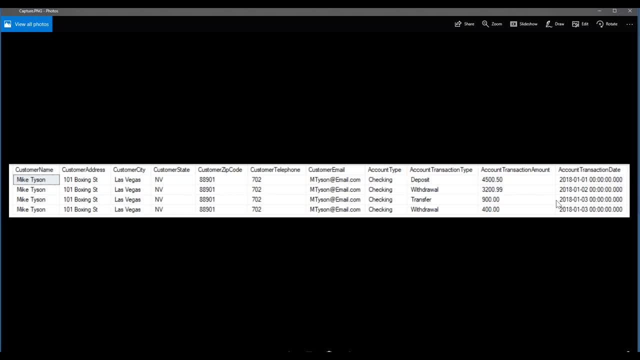 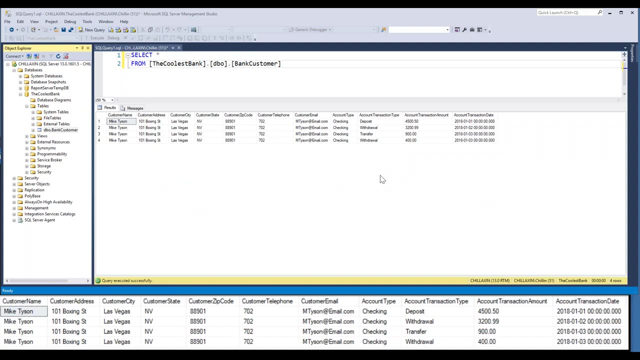 related to the account: The account transaction date. so this is more related to the account. And then there's a relationship between the account and the customer, because each account is owned by a customer. So now let's see how we can create or recreate this table into two tables. that's going to save. 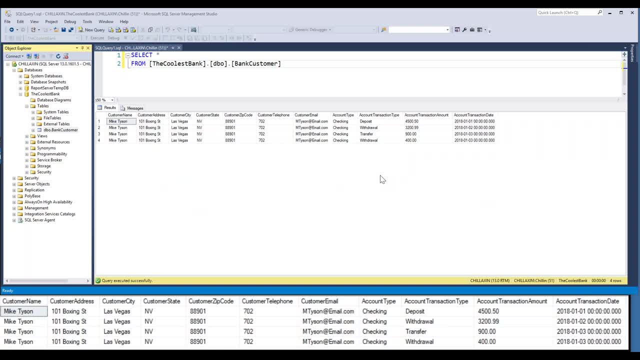 us Again. we can break it into more detail, but for now we're just going to simplify it and break it into two tables and see how that's going to help us in the concepts of normalization. So we'll go to our database diagram, create a new database diagram. It's the first time. 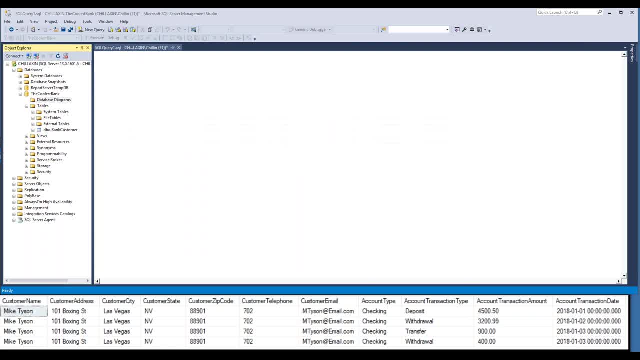 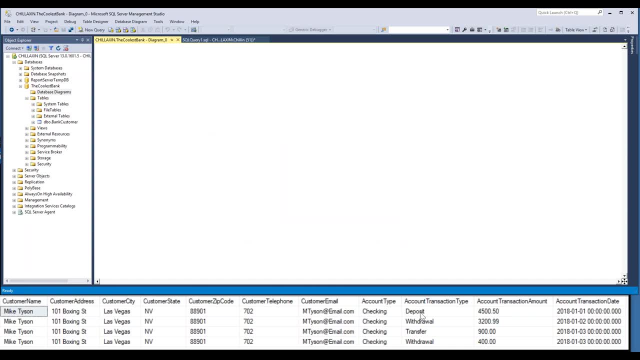 we're creating it, so we're prompted, We'll click yes. We're not going to add this table, so we're going to close, And we want to create two tables, one for the customer and one for the account. So right. 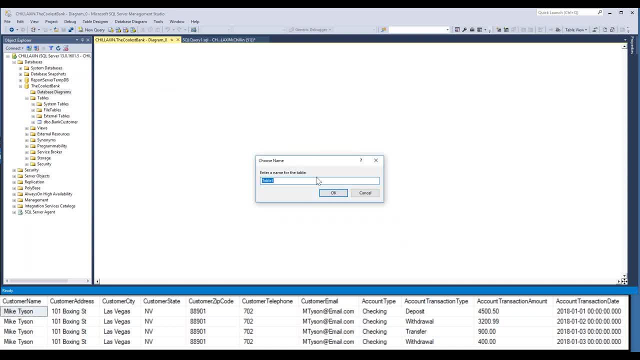 click new table. The first one's going to be the customer table And then the second table is going to be the account table. Okay, Rule number one is always Let's have the first column as a standard to be an ID column. 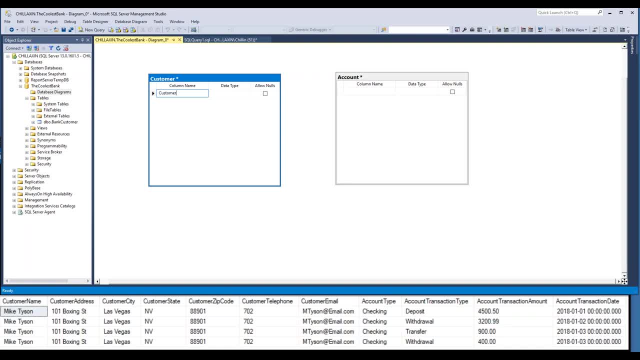 So what we're going to do is we're going to have a customer ID column and we're going to make it numeric, just integer, And we're also going to do something cool. So the first customer is No 1.. The second customer's going to be No 2.. The third one's. 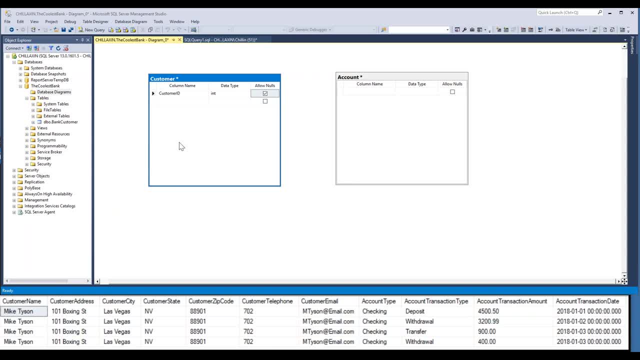 going to be No 3, even though that's not required here, but to kind of have our own little standard. It's going to be simple here. help us in the future if we need to query stuff or look up stuff or count stuff. so what we're? 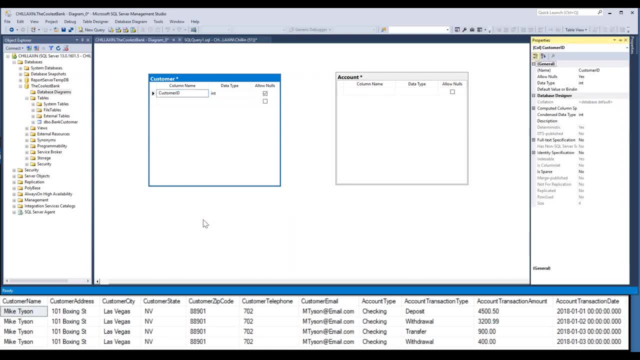 going to do is right click and look at the properties and then we're going to look identity specification. yes, so the first one is going to be employee number one and then it's going to increment automatically, so i don't have to enter the employee numbers or the customer numbers, as. 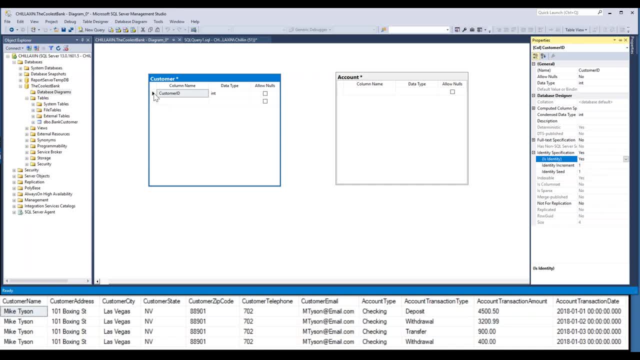 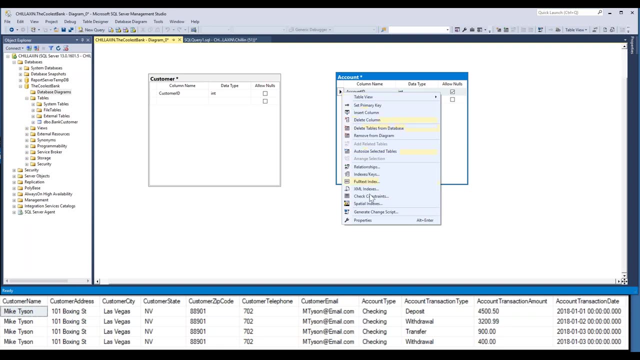 one, two and three, but it's going to keep incrementing by itself. and again, first column is going to be the table name id, so it's going to be account id. it's going to be an integer, so it could auto increment. we're going to look at the properties and, starting at one, incrementing by one. so now, 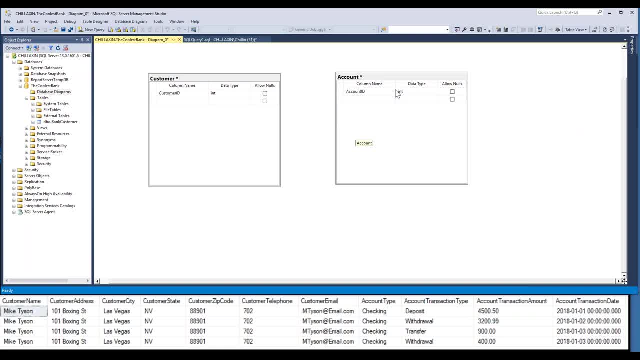 each time i enter account information, the first account is going to be account number one, the next one, number two and number three. all right, uh. the second thing is i want to make sure i have a relationship between this table and this table. so before i even enter any of those columns, let me go ahead and make sure i have a customer id. 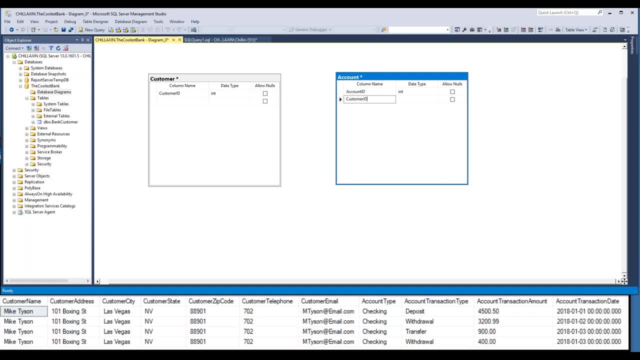 here. so i'm going to go ahead and add customer id as an integer and then we'll set this as our primary key on this table, and this is the primary key in this table and we want to create a relationship between this column and this column. so in here it's in state or in the 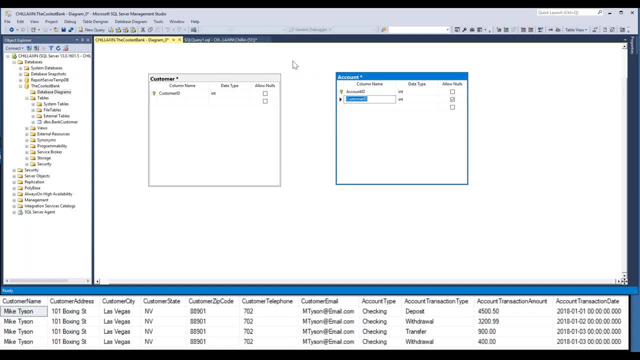 country or in the vicinity, so it's a primary key. but once it travels overseas it becomes a foreigner. so this is a primary key and here it's a foreign key. so when i drag, click and drag and drop it over here it's going to prompt me and says i'm going to create a new foreign key. 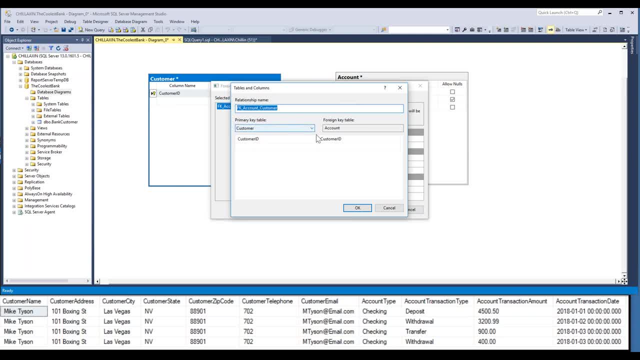 relationship: customer id on the customer table is a primary key, but customer id on the foreign key on the account table is a foreign key. is that what you want? yes, okay, and now i create a relationship between the custom id here and here. okay, now we can go ahead and enter that customer. 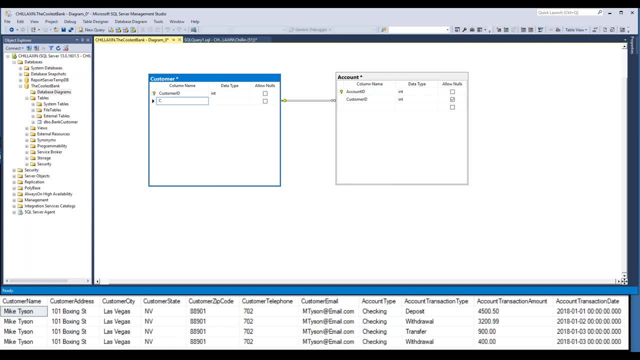 information. so we can enter the customer name- we'll do that as a varchar- and then the customer address. as a varchar we can enter the rest of the information. but for now we'll just run some of the other stuff, account type, varchar. okay, so at this point we have our customer table. that has the customer. 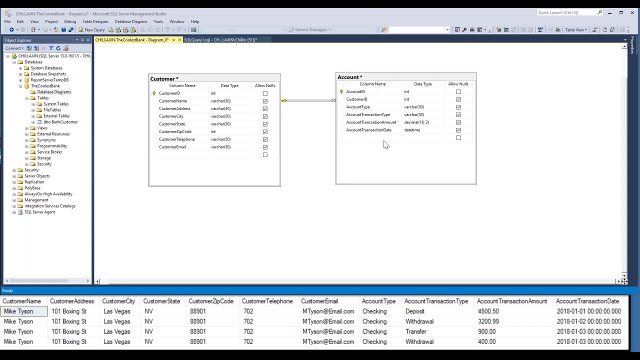 related information. we have the account table that has the count related information. we have a relationship between them, which is on the custom id, which is a primary key here and a foreign key here, and then each table has the first column is an id which is its own. 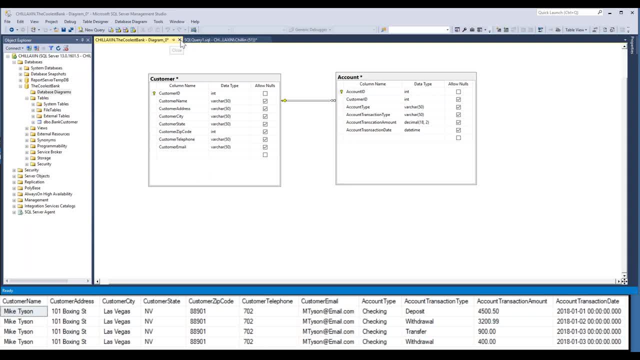 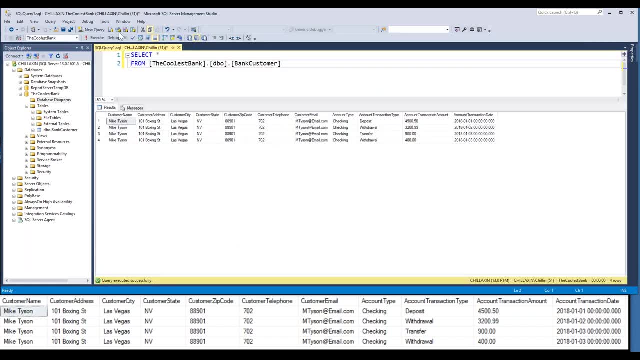 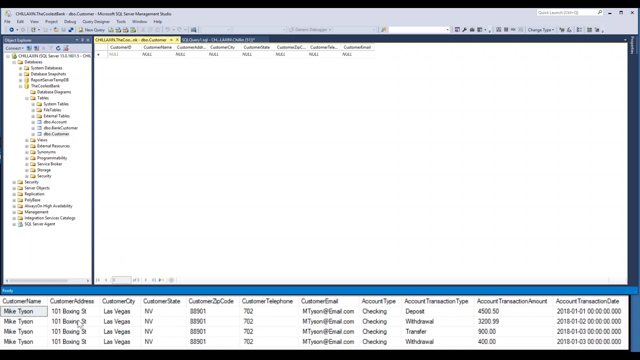 primary key. let's go ahead and create those tables. look, yes, so now we do a refresh, we should have our new tables. so now when i go into the customer table, i don't have to go into the customer table. i do have to enter the information four times. i merely enter it one time. 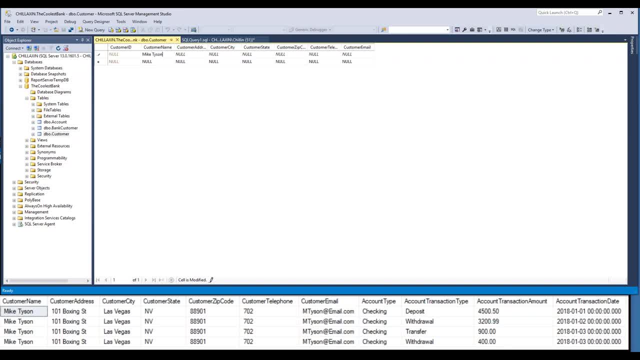 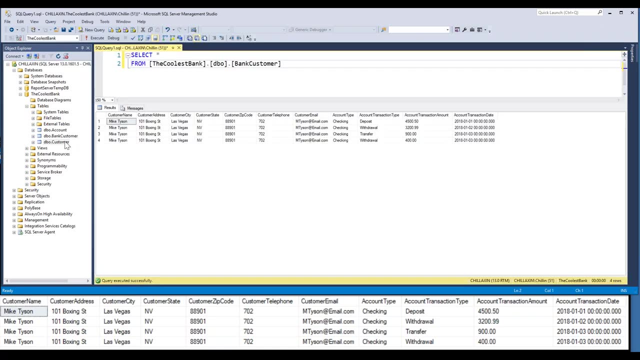 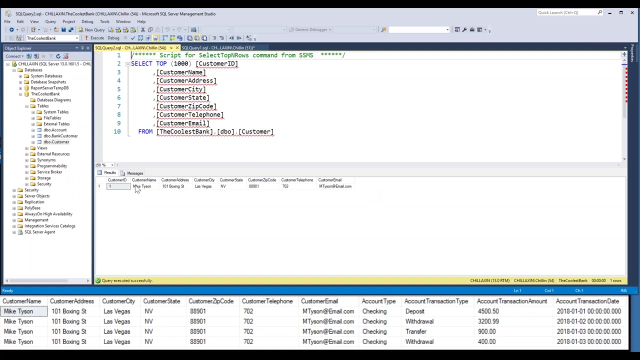 so notice, i only enter the information one time for mr mike tyson, and when i save it, of course customer id is going to be number one. okay, so number one. the information is just entered one time. next i'm going to choose varchar again and i'm going to go ahead and create my customer id. 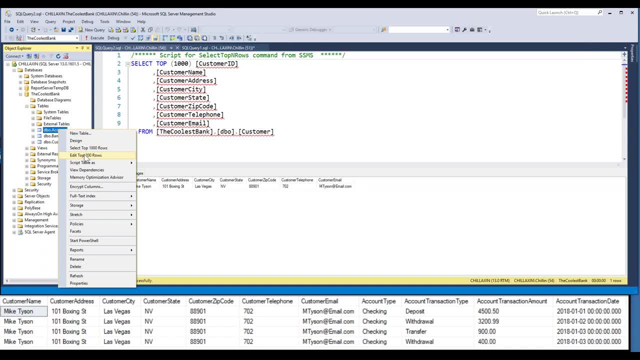 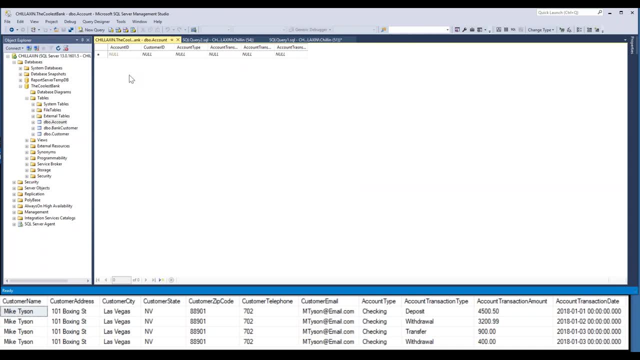 okay. so we're going to go ahead and create that new table and i'm going to go ahead and create your customer id. Now we can go into the account and we're probably, by the time we create it, are going to have four IDs for that information. 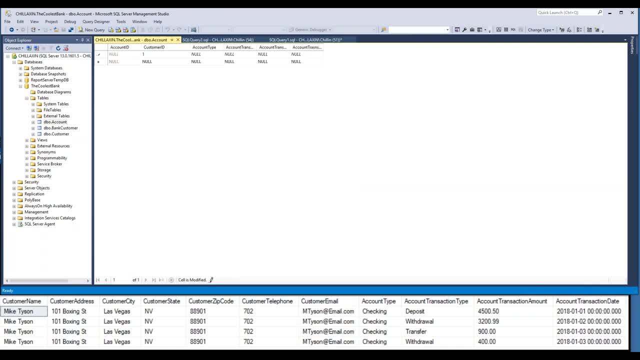 But then the account ID all I have to enter is one and it knows that all this information is related to customer number one, which is Mike Tyson. Now notice: for the account information, we've only entered customer ID number one, but it knows by default that that's all of this customer information. the customer name, address, customer. 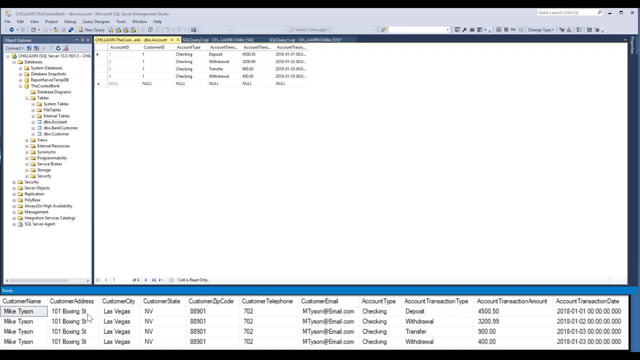 city customer state because there is that relationship as a foreign key. it's a primary key in another table which has all the details of it. So I don't have to no longer enter that information of name, address, city state, zip code, telephone. 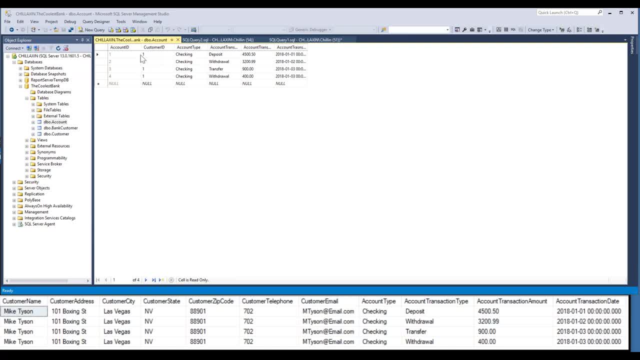 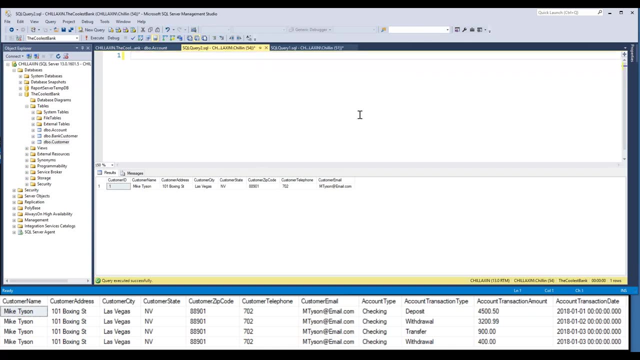 email and duplicate it each time. All I need is just a single reference of one, And it knows to get that information from my customer table. One thing that's really nice about having that relationship- a foreign key and a primary key in addition to that that's going to make our life easier- is I don't have to create. 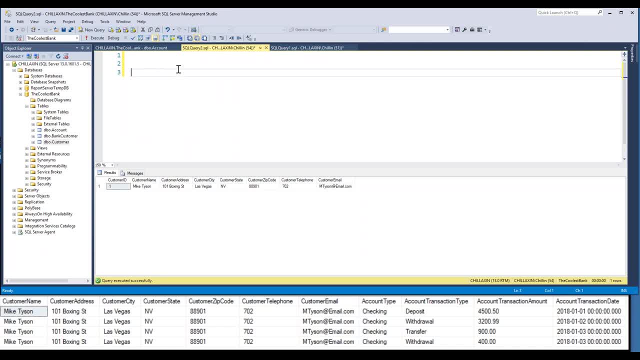 a select statement and build it. with the join I can have SQL Server do it because in the data dictionary it already has that information built in. So I can go to design query editor and say that I'm interested. I can get information from the customer and account table. 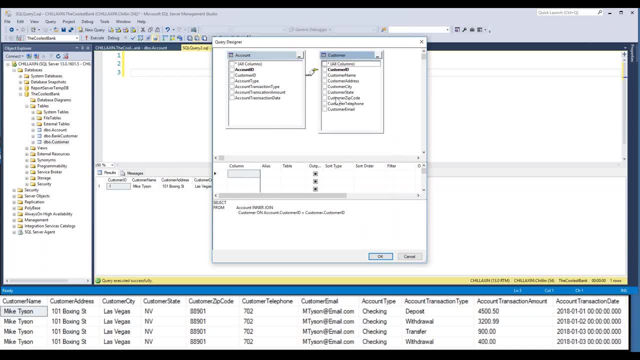 Notice how it automatically built that relationship because it already knows foreign key, primary key. So I want to get the customer name, their address, their city, their telephone number, and I'd like to have the transaction type and the transaction amount. So let's go ahead and check on those. 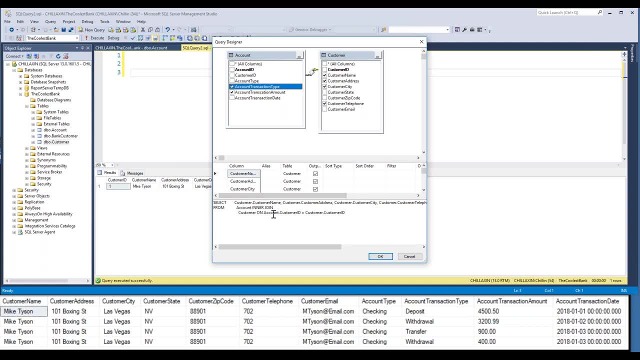 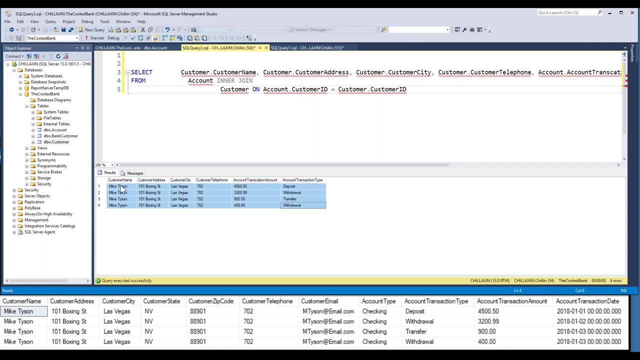 And it builds it for me because it already knows that there is a relationship on account customer ID and the customer ID in the customer table. Click okay, writes it up, execute and it gets me that information, Didn't have to duplicate it in data entry and waste storage and slow down my queries. 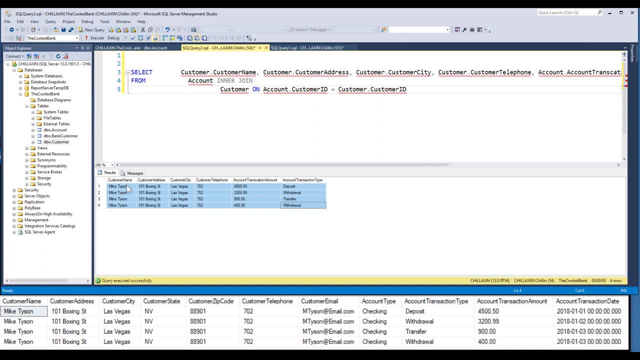 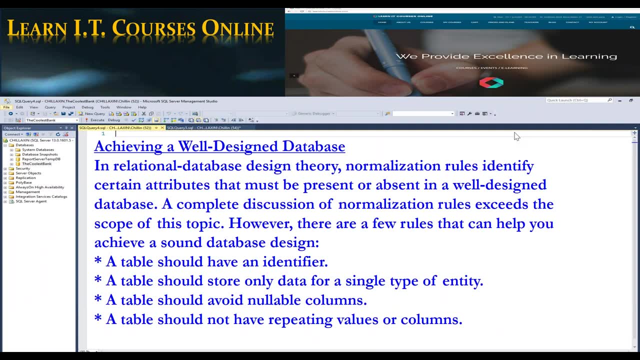 but when I query it, I can get that information in any format that I want, And that is what makes normalization very convenient and very beneficial. So now the mumbo jumbo that we talked about at the beginning probably makes a little bit more sense: that a table should have an identifier. a table should store only data for a single. 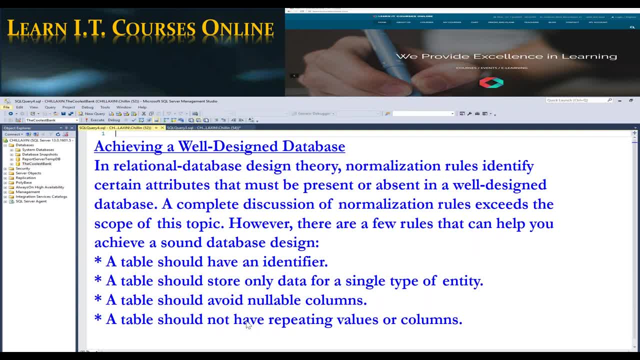 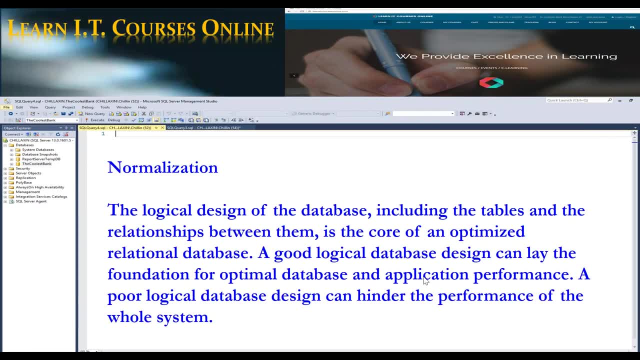 type of entity. a table should avoid nullable columns. a table should not have repeating values or columns, and that process of organizing it and designing it is called normalization, which is the logical design of the database, including the tables and the relationships between them. 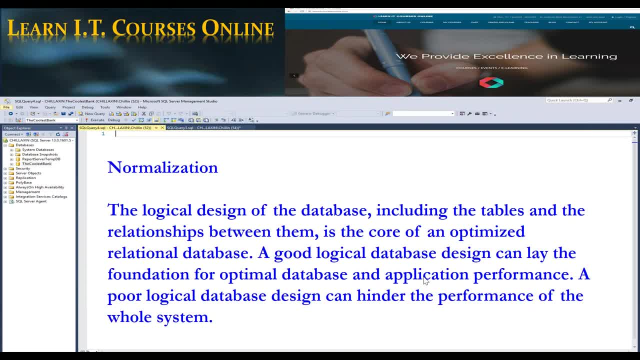 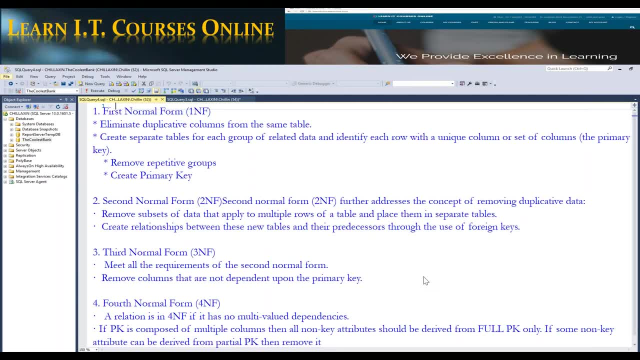 And it's the core of optimized relational databases. And then the four levels or forms of normalization, which includes, in the first one, eliminating duplicative columns, removing repetitive groups, creating a primary key. on the second one, remove subsets of data that apply to multiple rows of a table and place them in separate. 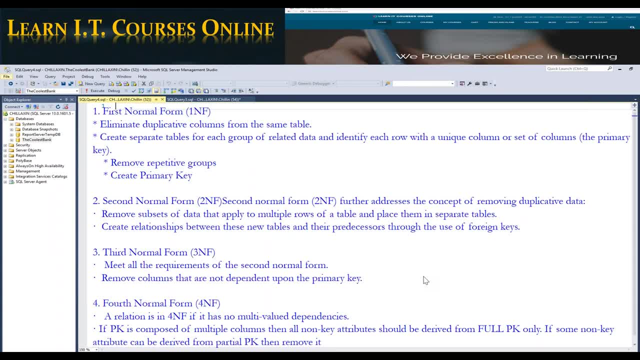 tables, Create relationships between these new tables and their predecessors Through the use of foreign keys. on the third one, meet all the requirements of the second- normal- But in addition to that remove columns that are not dependent upon the primary key. And then number four: if a primary key is composed of multiple columns, then all non-key. 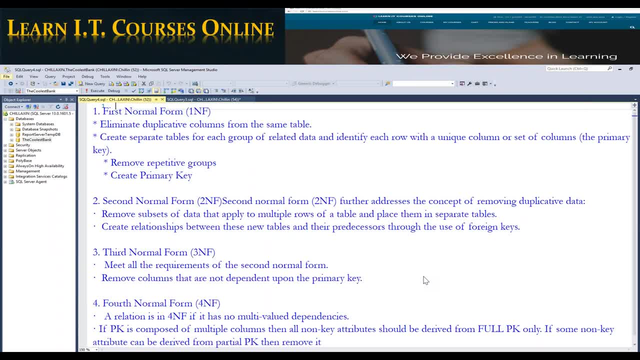 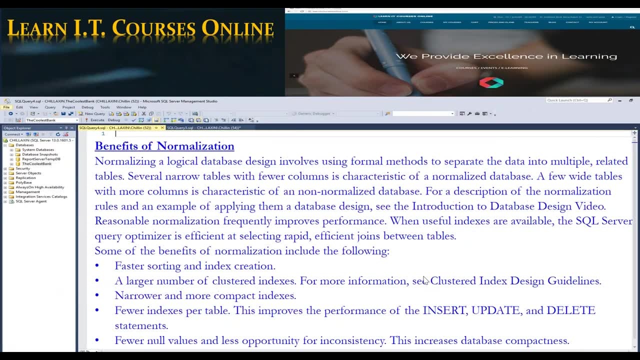 attributes should be derived from the full primary key only. If some non-key attribute can be derived from partial primary key, then remove them. And, as we said, there is a number of benefits of normalization, which include faster sorting and index creation, because now I have less data, a large number of clustered indexes.